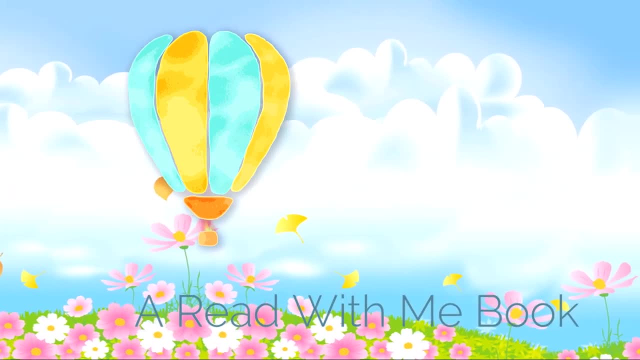 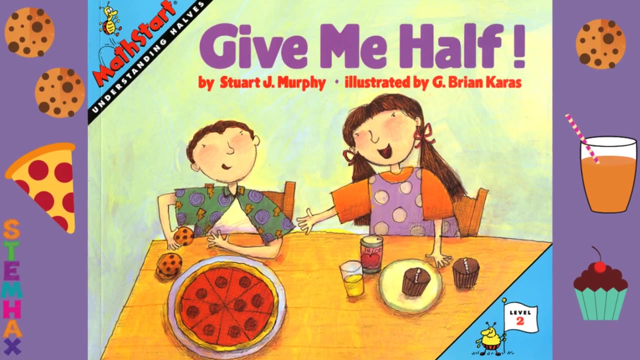 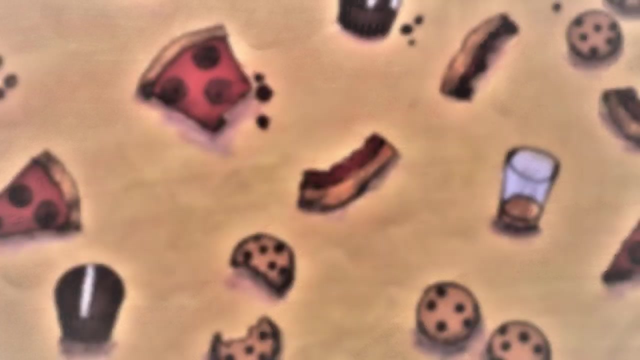 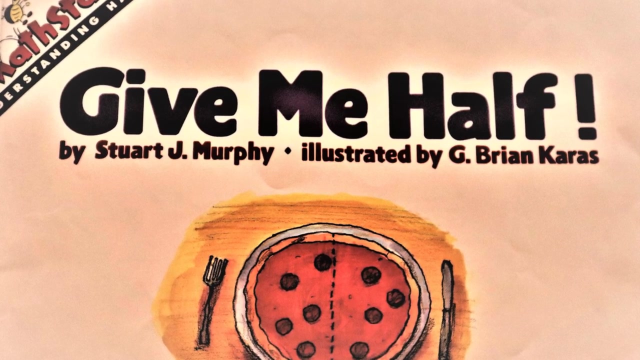 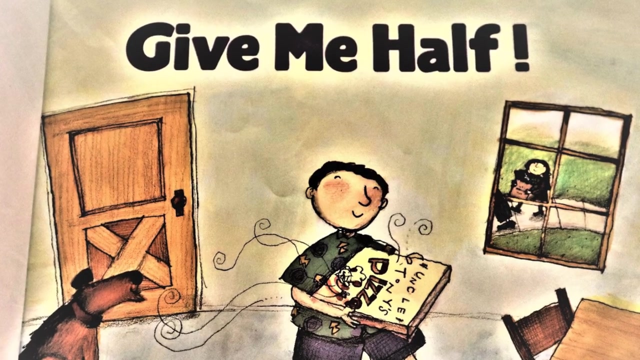 Give Me Half by Stuart J Murphy, illustrated by G Brian Karras. Give Me Half part of the Math Start series Understanding Halves, published by Harper Collins. Give Me Half. I have one whole pizza and it's all for me. 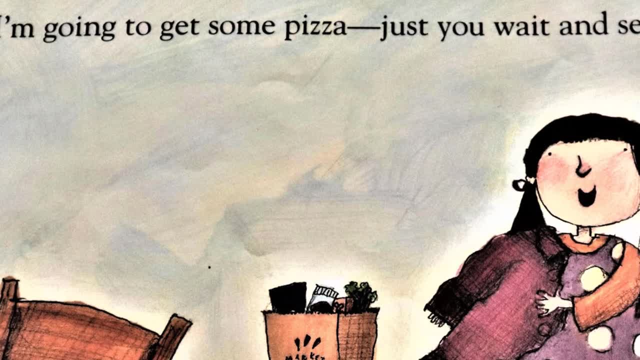 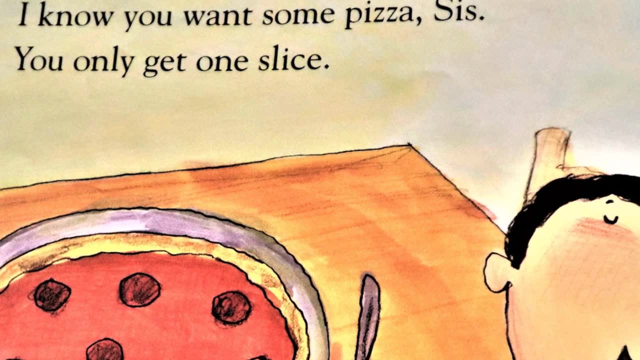 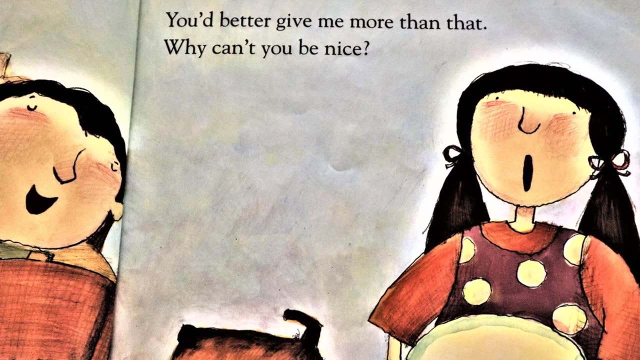 I'm going to get some pizza. Just you wait and see. I know you want some pizza. sis, You only get one slice. You'd better give me more than that. Why can't you be nice? You have to share the pizza. It must be split in two. 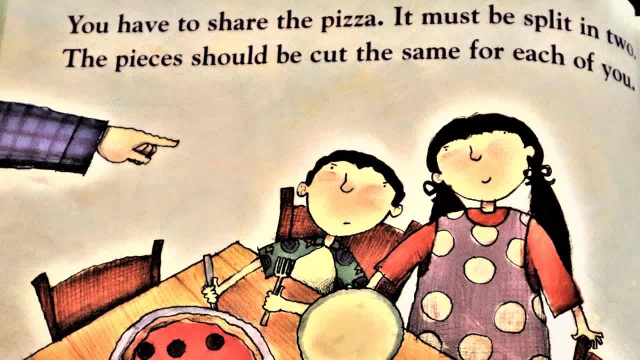 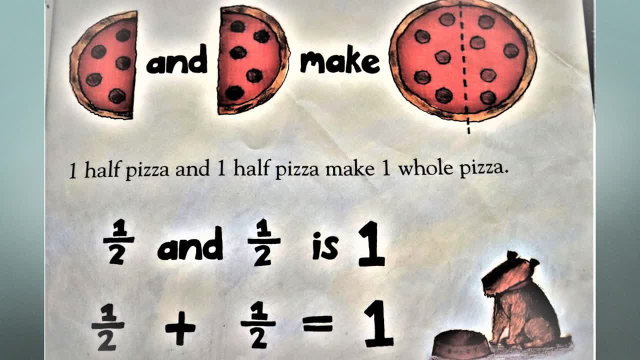 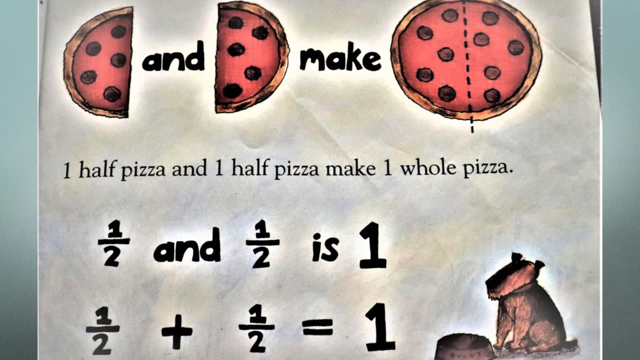 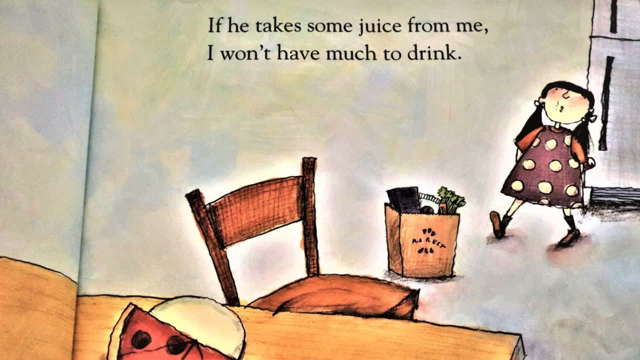 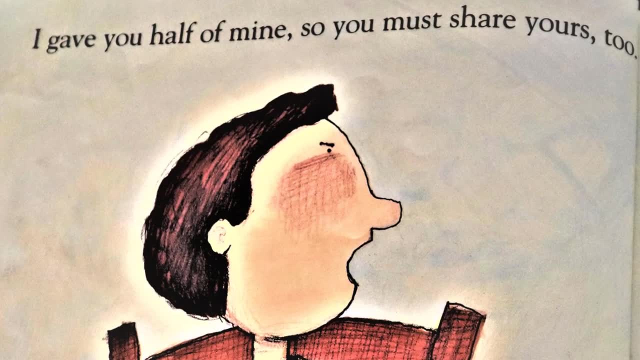 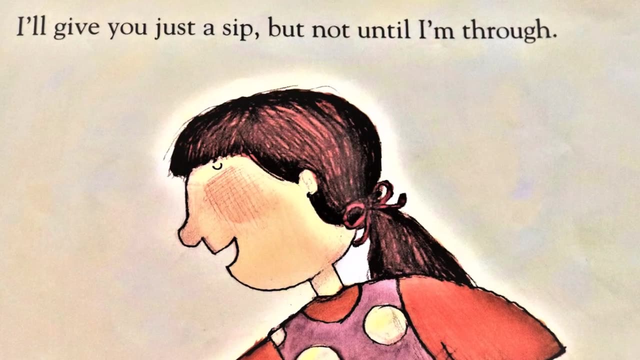 I think If he takes some juice from me, I won't have much to drink. I gave you half of mine, so you must share yours too. I'll give you just a sip, but not until I'm through. Split the juice in half Again. you have to share. 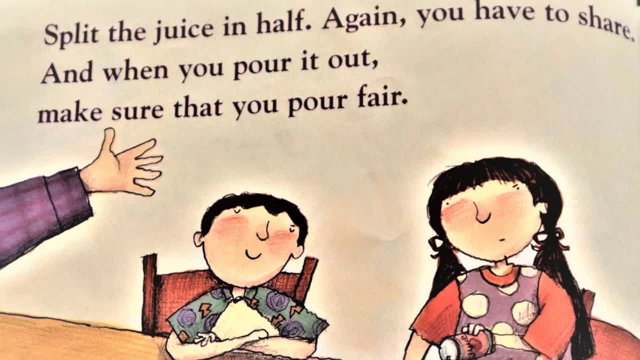 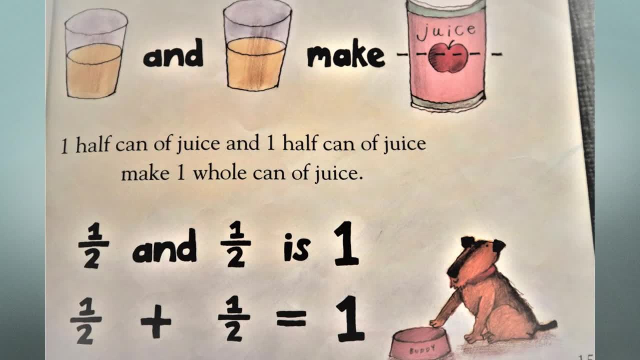 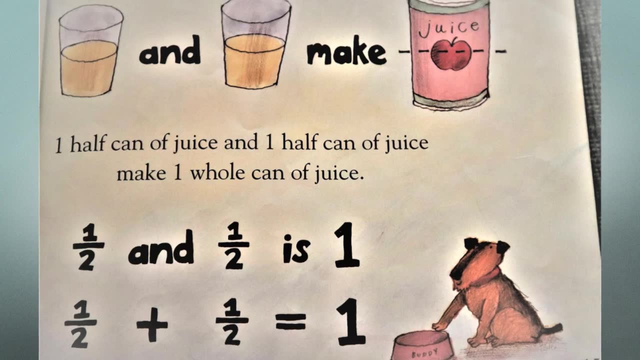 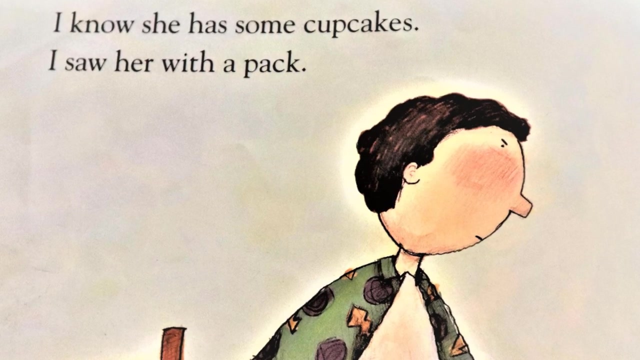 And when you pour it out, make sure that you pour fair. One half can of juice and one half can of juice make one whole can of juice. One half and one half is one. One half plus one half equals one. I know she has some cupcakes. I saw her with a pack.